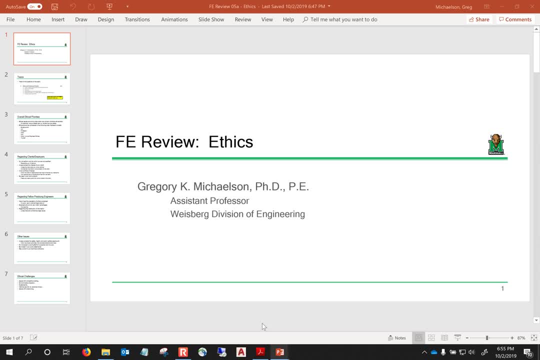 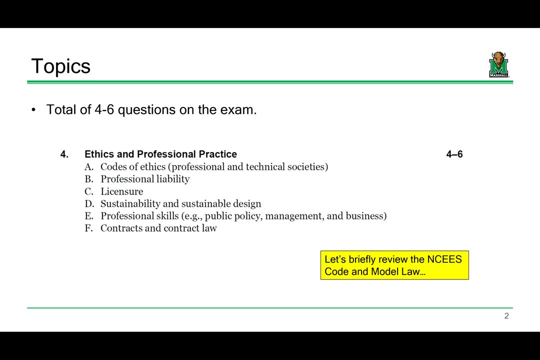 So with that, let's just go ahead and dive right into ethics. Let me pull this up, Okay, All right. So ethics, first off, is not a very big topic on the exam Anywhere between four to six questions, But it can cover a variety of different issues. 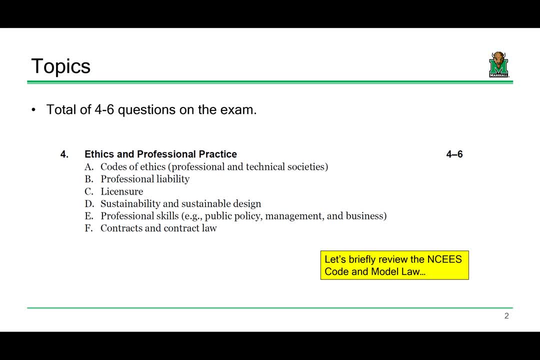 And one of the things about ethics is I really find it to be, I'd say, the most unique section on the exam, Because there's no computations involved at all, There's no equations at all, There's no values to plug and chug. 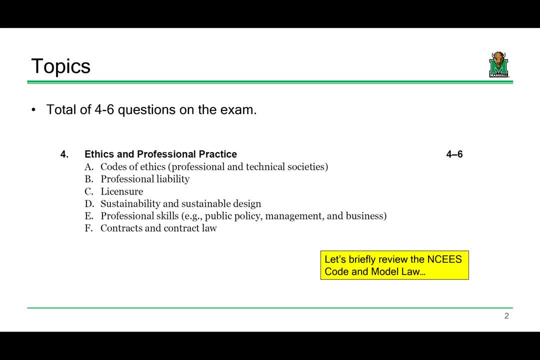 There's no units to figure out. It's entirely different, And so, as a result, I was thinking that our review should be just as different. Now, as for the list of topics that it covers, there's the codes of ethics, professional liability, sustainability, professional skills, so on and so forth. 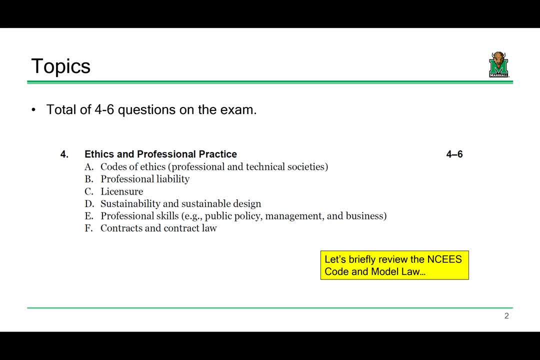 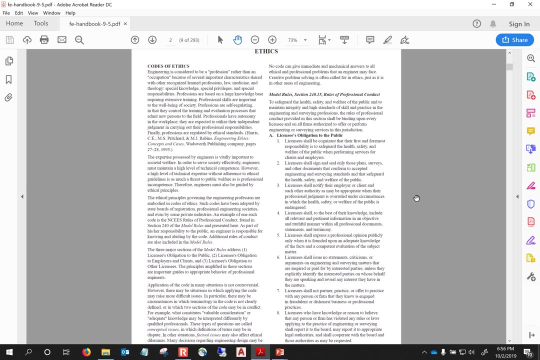 It really sort of boils down to your understanding of your responsibilities as an engineer. Now I want to briefly review the NCES code and model law, just so that you're aware. So I'm let me pull this up. So this is the FE reference handbook. 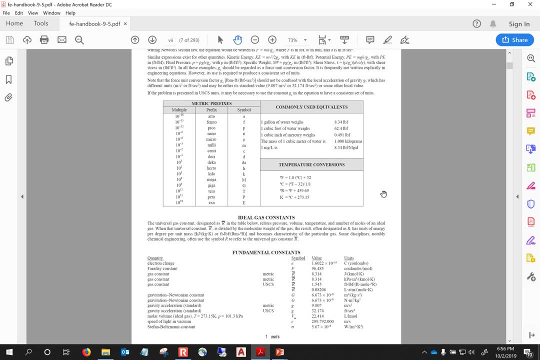 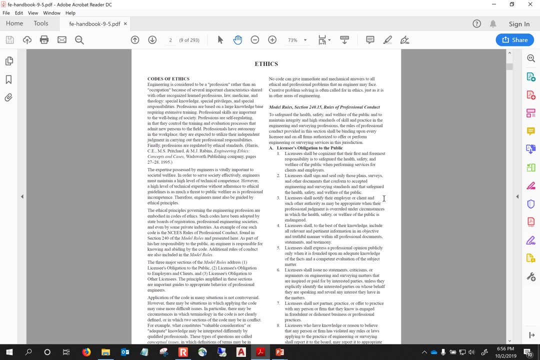 And it's actually early in the handbook. You know it starts off, there's units and conversion factors and things like that. And then the ethics code is actually quite early in the manual. Now it goes through and describes what some general provisions on the codes of ethics. 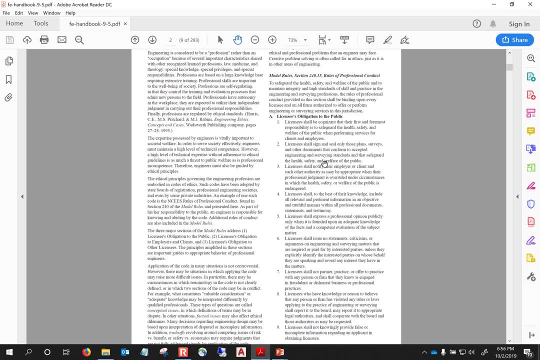 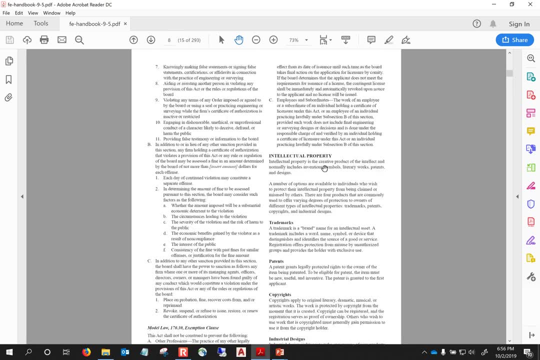 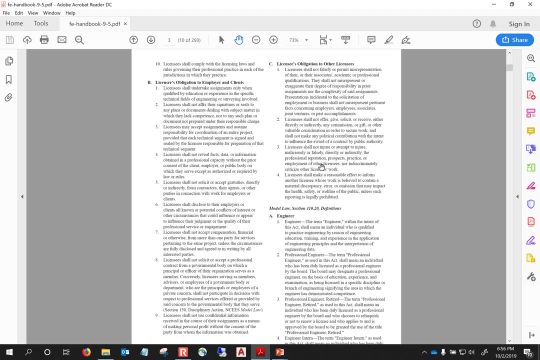 And then, if you look, it's actually somewhat long. It's, you know, I think, like four or five pages, And it covers, or actually more than that, and it covers quite a bit of different areas on intellectual property, trademarks, on surveying, and this, that and the other. 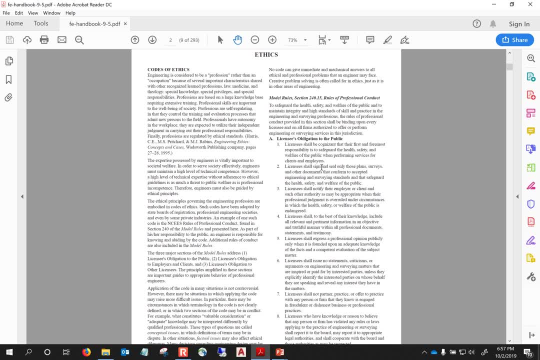 And it's a lot to take in. And it's also a lot- I guess the best way to describe it is- given an ethical situation for which you need to answer a question. it could sometimes feel like I don't know where to look and I don't know where to begin. 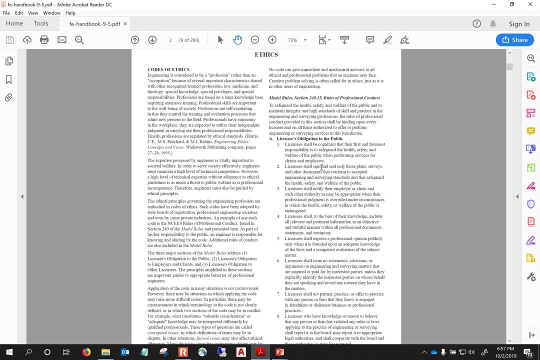 One of the things you will find with the ethical questions that you get on the FE exam is that there is a clearly defined answer. You're not really asked what I call gray questions On the exam. they might seem gray when you first read it, but there is a clearly defined answer. 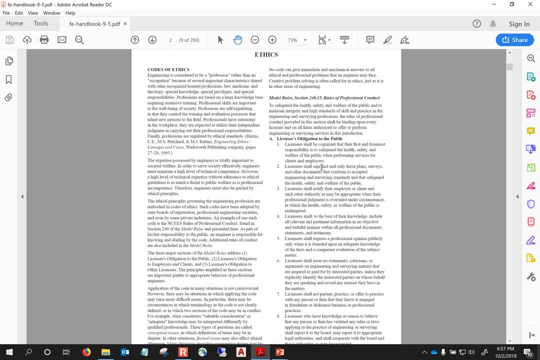 And that answer does tend to refer to one of these provisions. But because there's so much here and there's so much to take in, what I've decided to do is sort of boil that down into what I think are the most critical provisions that I think you need to understand. 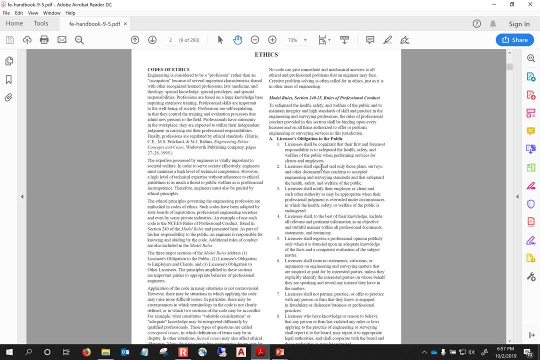 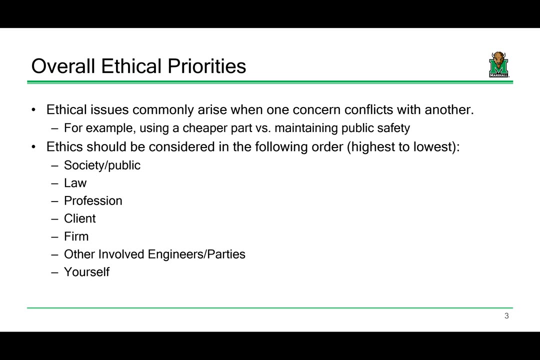 And sort of, I guess, Some of the common pitfalls and the common ethical challenges that engineers face. So let me get right into that with this presentation. It's somewhat short but I do want to discuss some of these issues in detail. So first off, let's talk about overall ethical priorities and where ethical challenges come from and where you know some of the questions that you're going to get on the exam and common ethical issues that engineers face. 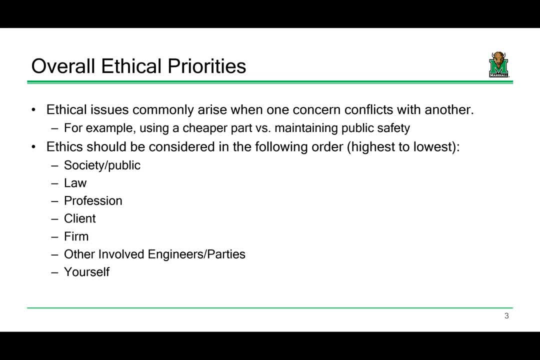 It always happens when One ethical responsibility or concern conflicts with another. So just to frame that in a very simple, easy to understand challenge, let's say you had to make a decision between using a cheaper part or a cheaper beam, or a less expensive product. 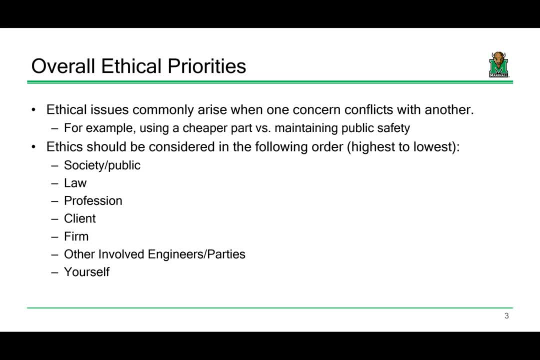 But using that product or implementing that part could cause an issue With public safety. you know, if I, if I have an engine and I put a crappy gear in it- pardon, pardon the term- but I put a bad gear in it and the engine blows up and hurt somebody, that's an ethical challenge. 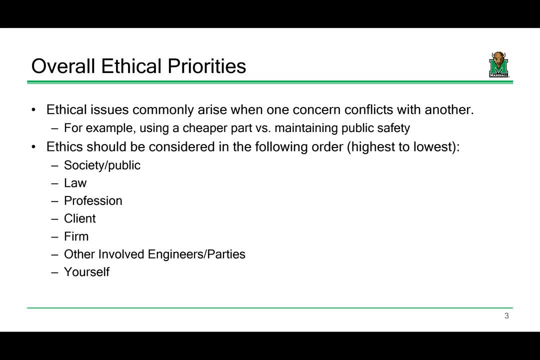 So what do I do? Do I use the cheaper part and save some money, or do I use the expensive part and ensure that the public safety is maintained? Well, that's pretty easy. I think that's a pretty straightforward: use the gear that's safe, even if it means. 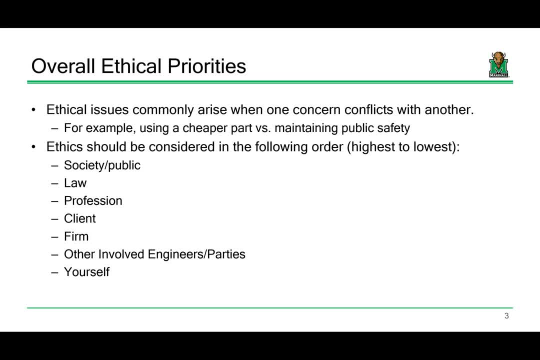 Uh, it's more money, because the safety of the public is your primary concern, right, That's easy. Well, that's an easy one. Sometimes on the FE might get one. That's not so easy. So where do you rank your, your priorities? 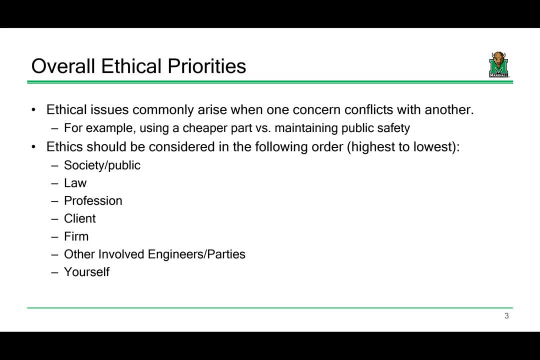 Well, so here on this slide I have what the engineers priorities are, in order of. you know, what's the most important to what's least important. So, the first off, what's most important is society and the public, And generally what I'm talking about there is their safety. 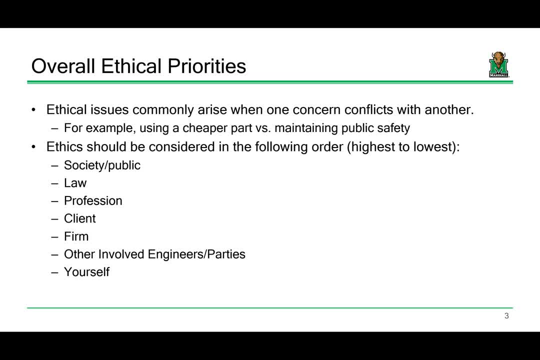 You cannot design anything that is unsafe or that poses a risk to the public's welfare. It's your primary concern And right off the bat. if you're ever having a question on the FE and there is a choice that would cause a, there is an option that would lead to a detriment of the public safety. it's the wrong answer. 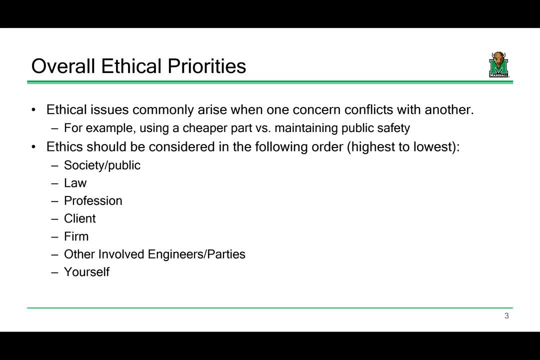 Just right off the bat: Um. next comes the law- Engineers must follow The law- and then uh. next comes the profession: uh, then the client, uh and your firm, uh, and to the client and the firm. that things like that relationship can get, uh is where a lot of potential ethical issues can arise. 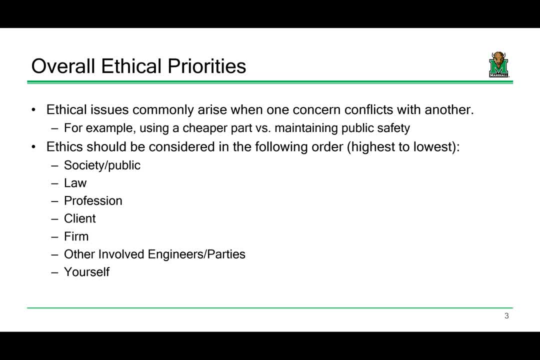 And we'll talk about that here in a little bit- uh, other involved engineers, other involved parties and then finally yourself. uh, and that's sort of another point with ethical concerns is that your first Primary concern is the general public's welfare and safety. 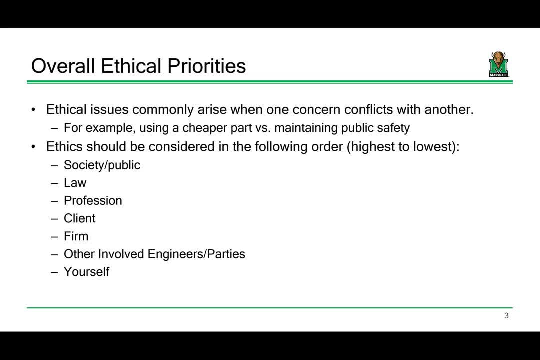 The last concern is yourself. Um, your, your, your priorities are last on this list, Um, but excuse me, um. what we're going to do is, I think, that's pretty easy to understand. However, what I think is a little more challenging, I would say, is, is some of these, these topics in the middle. 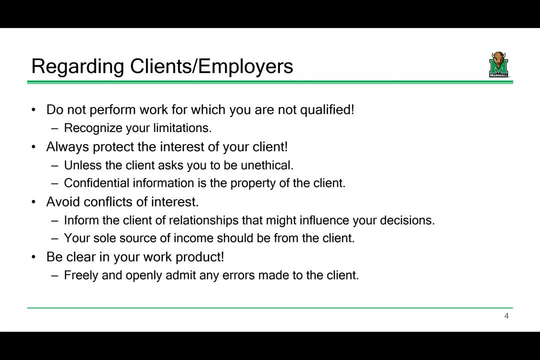 So let me go to this, this next slide, and I want to take some of these issues And and, one by one, boil them down. So, first off, I have some points regarding your client and your potential employers and- and these are some high level bullet points- 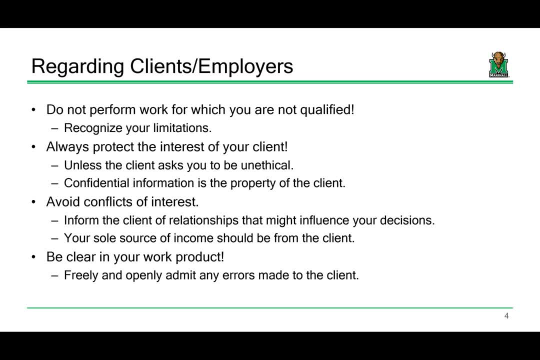 I think you need to keep in mind. First off, do not perform work for which you are not qualified. Okay, Um, and there there are a number of potential questions you'll get on the FE where it's leading to that uh topic. 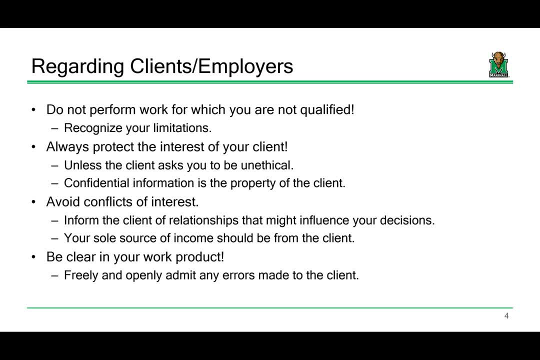 Um, you will never see me Design a circuit. I am a bridge engineer. I wouldn't know the first thing about it, So I know that that is not within my technical area and I'm not doing it. Um, recognize your limitations. 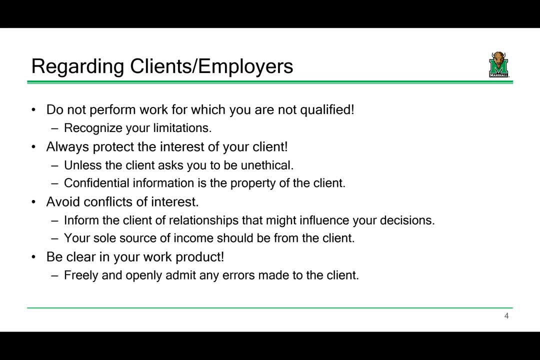 There's nothing wrong with that. Um. you have a given skill set. That skill set is your area. Um always protect the interest of the client. You are working for the client, so their interests should be your primary concern, unless the client asks you to do something that is unethical, in which case you can't do that. 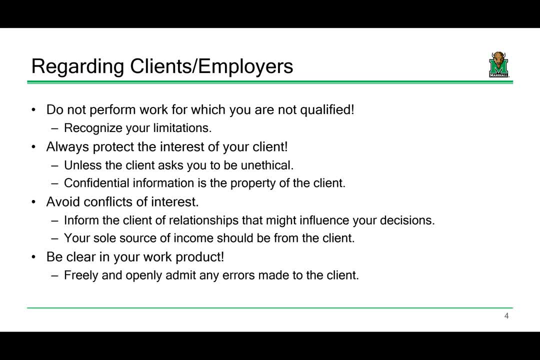 You're working for a client and you know, let's say, they're an industrial manufacturer- they produce, you know uh, some sort of industrial uh client and they ask you to falsify, uh uh a water quality report that they won't get fined. 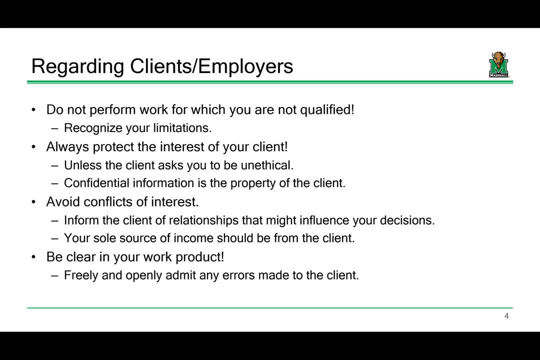 Yeah, you can do that. Okay Um, recognize uh this. this next bullet point, um, I think can can lead to a lot of pretty straightforward answers on the exam. Recognize that any Okay Um, information that is to be considered confidential is not your property. 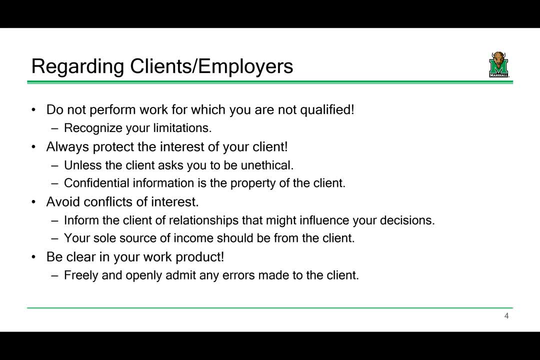 It is the property of the client. The client owns that information. So whenever issues of confidentiality arise, if you keep that in your mind, I think that a lot of potential challenges uh can be met by just recognizing that that primary concern. 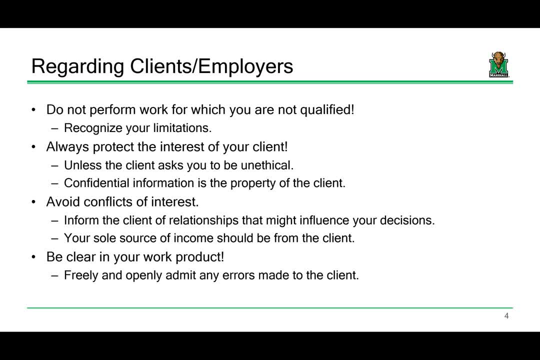 Um, avoiding conflicts of interest. So I'm a bridge engineer, so I'll give you a bridge engineering example. Um, um, let's say that there is a company that creates a new type of reinforcement for reinforced concrete using some sort of uh advanced polymer. 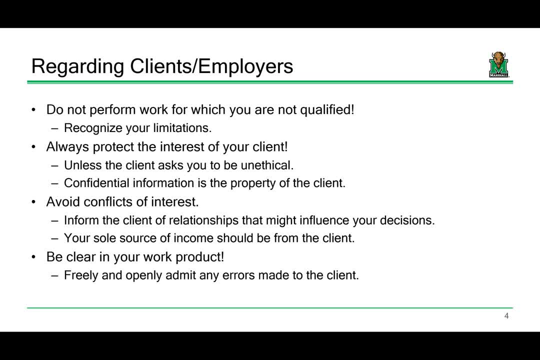 And I think that this is going to revolutionize the market, so much so that I personally invest some of my funds in a company manufacturing this stuff And then a project comes along where I want to. I need to design a bridge And I use that reinforcement, even if it might be the best product on the market, even if I believe that I have a financial interest in using it, because the more that that product's used on potential money I could make. 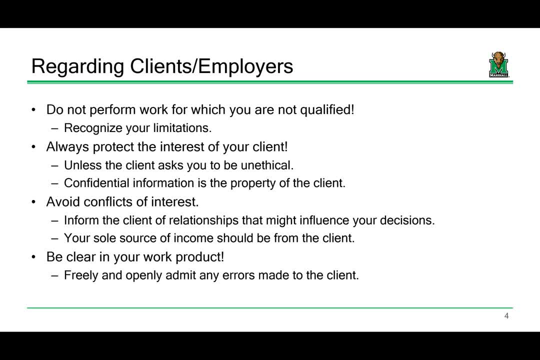 So there are some very uh significant challenges there. Um, make sure that that you're informing your client of any uh relationships, investments, anything like that, that could influence your decision. uh, because otherwise you would be misleading your client. 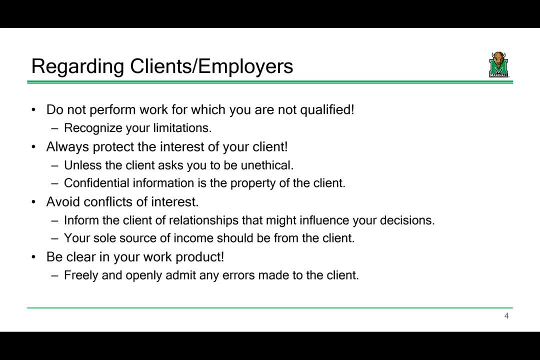 And so, and, and you need to keep that uh relationship paramount. And so your sole. another way of thinking about it is that your sole source of income or compensation, or or, or what have you from a particular job should be whatever fee your client is paying you. 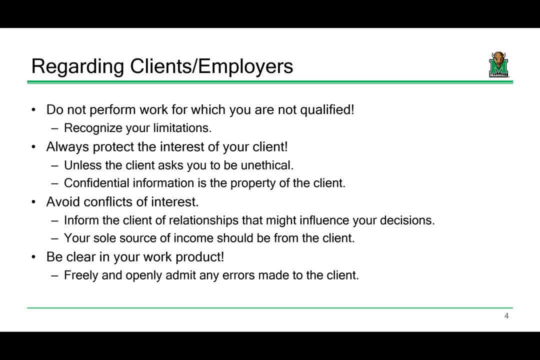 And that's it. So, if, if you keep that in mind, I think that that again, a number of those issues on the FBA will be resolved. Um be clear in your work: product. Um, engineers are human beings. 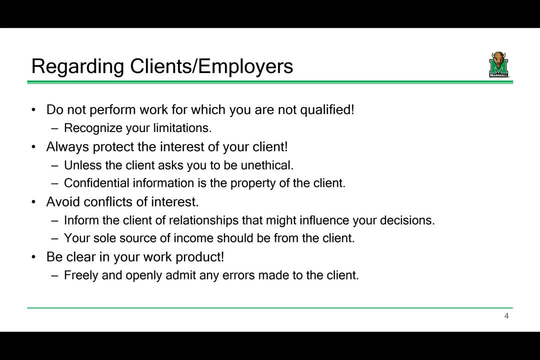 If we weren't, we wouldn't need to have this discussion and all of this would go away. because you're a human being, You can make errors as possible, openly and freely. admit those errors to your public Do not- or to your client. 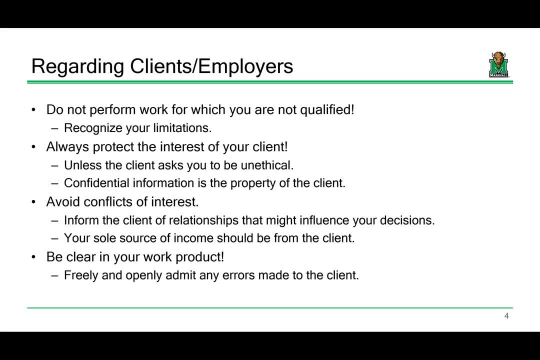 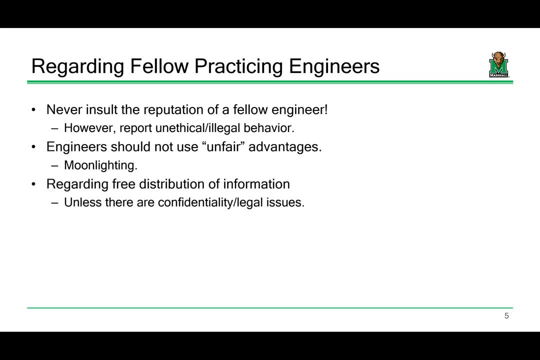 Do not conceal that That will cause very significant issues down the line. Okay, Okay, Regarding your fellow engineer, um, ethical issues that can um arise regarding your peers. Okay, Never insult the reputation of a fellow engineer. Um, there are, uh, a number of project specific pieces of information that you might not be privy to. 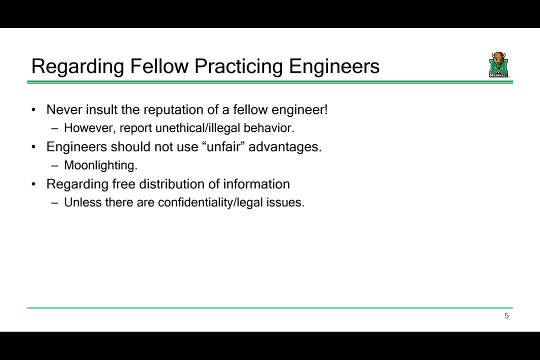 Uh, and and unless, um, unless you're aware of this could cause an issue. I'll give you an example, And again, I apologize if I point too much to the bridge engineering world, but it's what I know: Um, for example. um, let's. 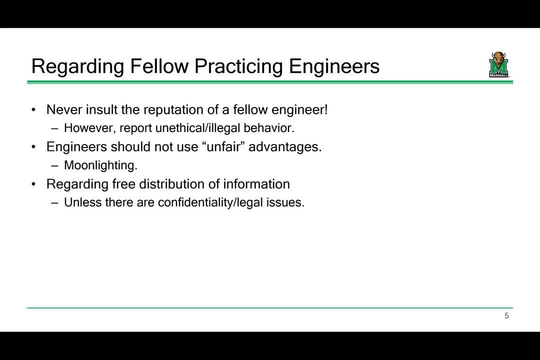 Let's say that I'm looking at a bridge design and I see their, their beam design, and I and I do the math and I realize that beam looks a little over designed and I might think to myself, well, I might start to get a little critical of that engineer, but there might be a host of other issues that I wasn't aware of that cause that engineer to make that decision. 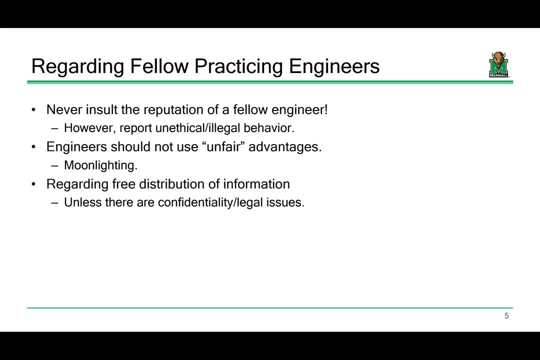 Maybe there were sourcing issues, maybe- um, maybe there were there were- uh, it it. by picking that beam, The lead time Uh was decreased substantially and it ultimately decreased labor costs and decreased the cost of the project. 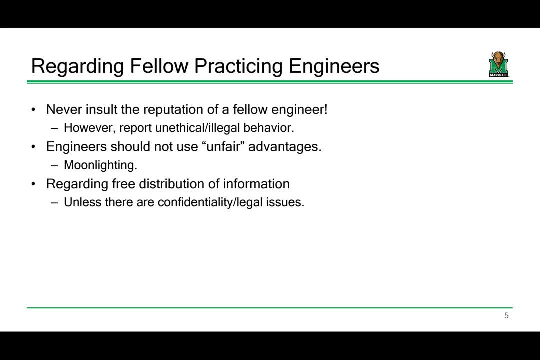 Um, decisions like that happen in bridge engineering all the time, uh, and in the end lead to a more economic product that doesn't compromise safety at all. But then again, all I'm doing is looking at the plans and here I go wanting to make um, uh, uh, sort of these, these criticisms of the engineer, without understanding all the facts. 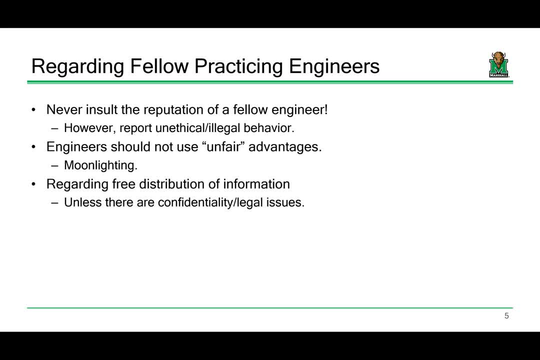 Now to be clear: if, if you have reviewed a design, Uh, or or reviewed something that you believe is an ethical, that is gonna uh lead to a, a, a challenge to public safety. If you believe that you, uh, you know, uh- discovered a legal behavior, well, of course, you need to report that. but this is one of the the reasons that that we- we had this ethical provision, because, without having all the facts, you aren't aware of what's uh, what's going on. 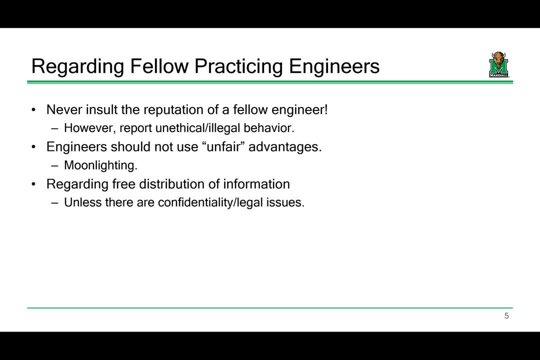 Um, engineers should not use unfair advantages, and so one very common Uh topic on the FE exam that might pop up is the idea of moonlighting. So what do I mean by moonlighting? Well, let's say you are a salaried engineer and you know you work a, a, a, a full-time job and are paid on salary. 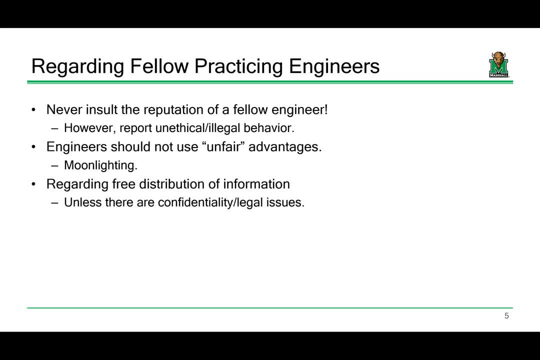 And then at night you decide well, or in your spare time you decide well, I'll do some consulting on the side. Um, and that's a, that's a gray area. Uh, and honestly, many engineers do that. 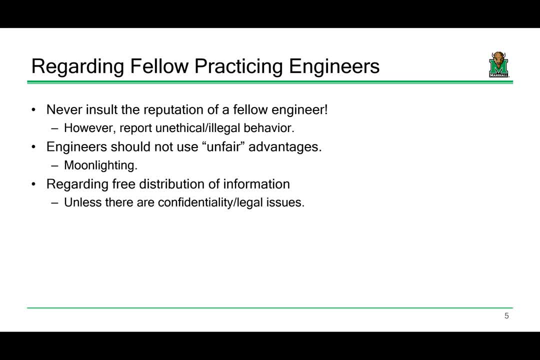 The only um really where the ethical issue comes from is when you're engaging in behavior that puts you in an unfair advantage. In other words, you're doing work that other engineers and other peers in your field couldn't do. They couldn't take, uh, those advantage, uh, those uh uh, they couldn't take those advantages. 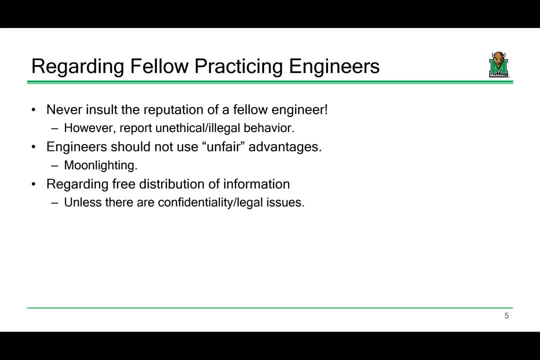 That's. that's where the the ethical issues arise. So moonlighting is something That, uh, you would definitely want to avoid, And if there are allusions to moonlighting on FE exam problems, it will generally be regarded as an unethical practice. 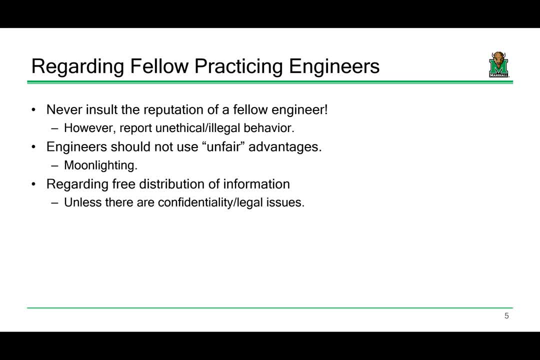 Um, now here's another thing about, uh, regarding your peer engineers. Um, engineers should um generally promote free distribution of information. We want to improve the profession, And so the way that we do that is when we discover something or design something. 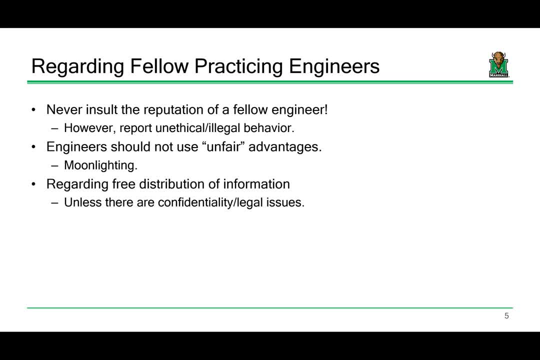 And, and as long as we're not violating confidentiality issues and things like that, that information should be widely available to the public. Um, for example, um, uh uh, research and understanding on a given phenomenon in engineering. uh, engineers should want to make that available if it's gonna improve the profession. 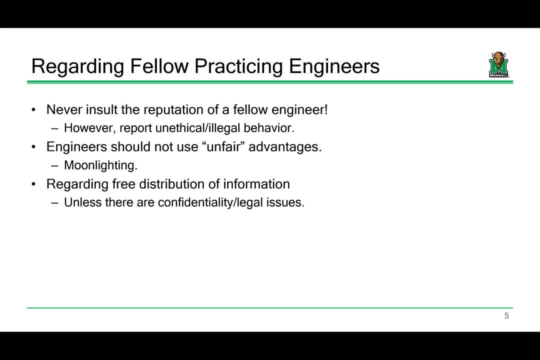 Now the. the limit to that is when those issues start to bump in the face of client confidentiality or legal issues or things like that. I'll give you an example that's actually not bridge related. let's look at the building design sphere. one of the more complex areas in building design is to design. 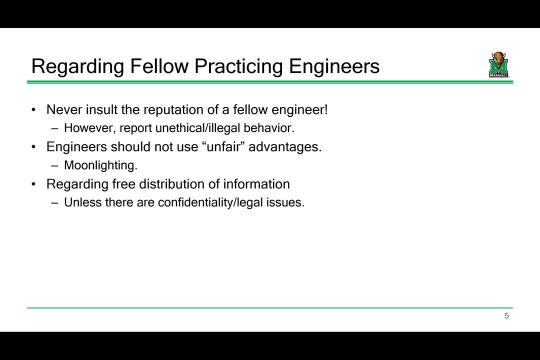 for seismicity or earthquakes and it's a very complex field in structural engineering and, as a result, there are many different proprietary systems that are out there in order to to arrest seismicity. so the general idea: you have a building, you excite that building with an earthquake, the building wants to. 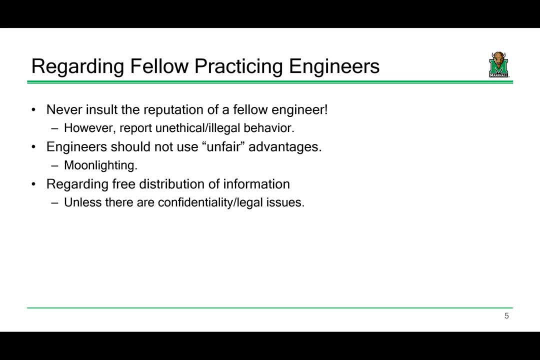 displace laterally and it will undergo large deflections and will experience a large amount of forces. and so, as long as the building remains upright and and people can get out safely, that's the one of the primary focuses or goals of seismic design. and so there's all sorts of proprietary bracing elements and racing systems and 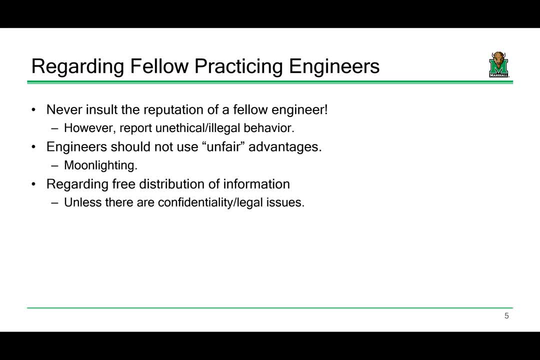 things like that out there that are available for engineers to use. now their there are plenty of companies- andemic and fabricators and things like that- that are developing systems, and there are some elements to the systems that are proprietary. everything else so about this system is made available to the. 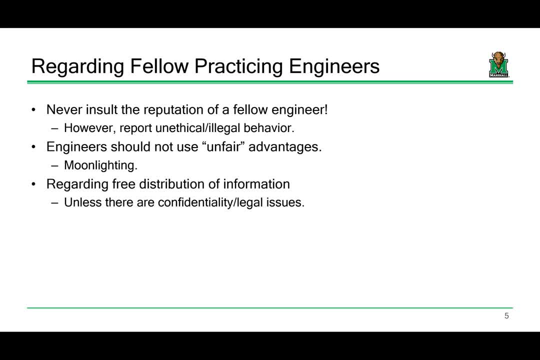 engineering community. for example, if you're a company and you've designed a new type of work technology which cannot be sold anytime soon as you're holds an of brace that you can install and steel frame that has so and so or has such, you know, improved performance under earthquakes, well, you're going to want to. 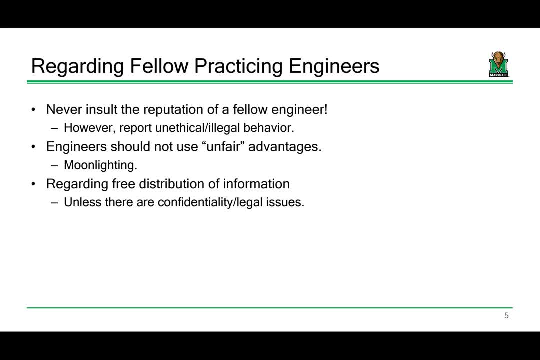 tell the engineering community all about its performance, make sure they understand the hysteresis behavior, that they know what our values would be applied, and so on and so forth. and the reason is is because engineers need to know that in order to be able to implement it. that doesn't mean that you 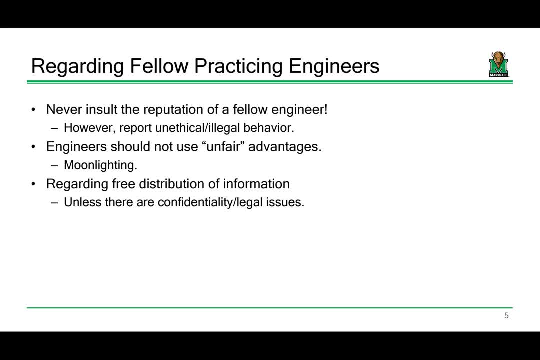 need to explain every single little aspect of how that is fabricated. there are plenty of elements like buckling, restrained braces, where, as long as the engineer understands the predicted behavior, they can make that decision, but the proprietary aspects can still be protected. so just something to keep in. 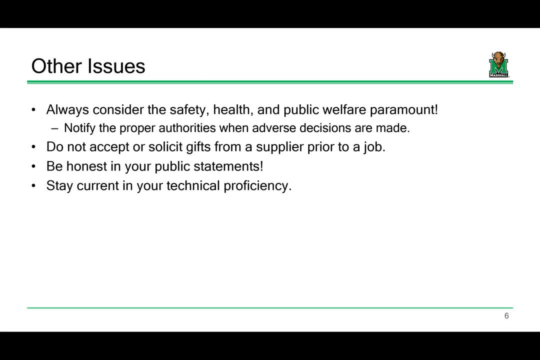 mind some other issues that can arise, just not only with ethical issues, but just things that you need to know about the structure of the structure of the structure that you can see on the FE exam. first off, again, like I said- and this is a dead giveaway if you ever asked a question on the exam where a 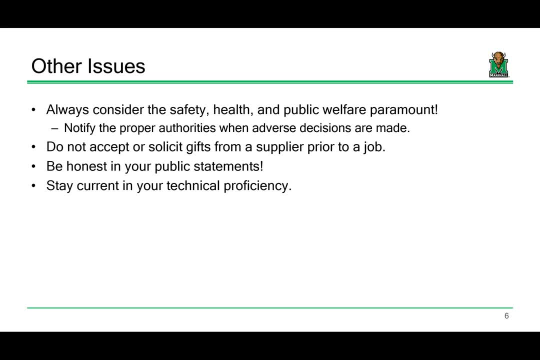 choice would compromise public safety. it's the wrong answer. okay, always consider the safety, health and welfare of the public as paramount. if there are ever any, you know observations that you make where an engineer has compromised public safety, you should notify the authorities. that practice is called whistleblowing. ironically, that terms 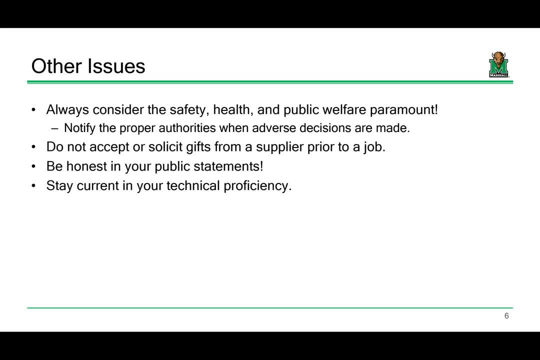 floating around the news right now. but in regards to engineering, what I'm saying is when you observe a practice that could put people in danger and you report that to the authorities in the engineering sphere. that's what I mean by by whistleblowing, and whistleblowing, to be clear, is fine if you're doing in. 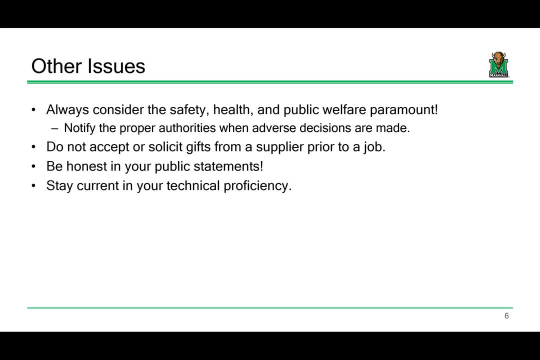 it to ensure that the public safety is maintained. it's actually you have to do it. don't accept or solicit gifts from a supplier prior to a job. you're an engineer. some bean supplier slips you tickets to the Super Bowl so that you'll use their beans. yeah, that's unethical to take that. so that's a pretty common type. 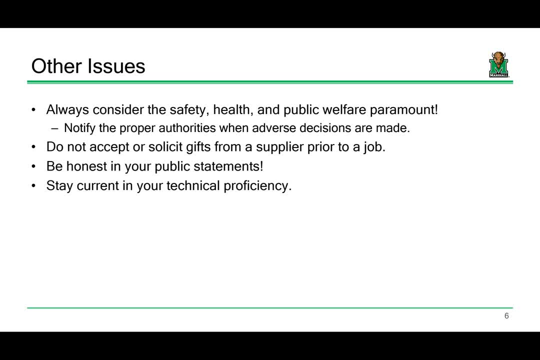 of question that you would get on the exam. be honest in your public statements. if you're ever making statements, be completely honest. make sure all the facts are are made aware of. that's fairly important. and another thing: stay current in your technical proficiency. this is it's something that I've even 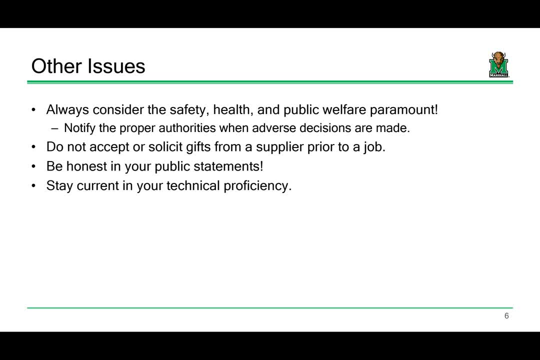 personally seen happen and kind of bugs me a bit. I you know you go to a conference and there are engineers that are attending presentations so that they can collect their PDH's for licensure, for to renew their professional engineers license, and they're clearly not paying attention. 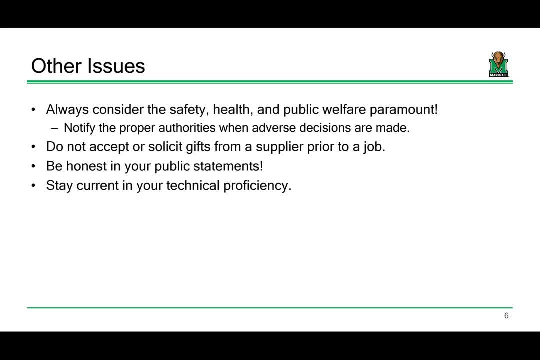 they go in to the room, sign in and leave and then come back later and pick up their certificate. that happens quite regularly and that's not really doing you or the public any good. being current and being up-to-date in the practice of engineering does you good, does your? 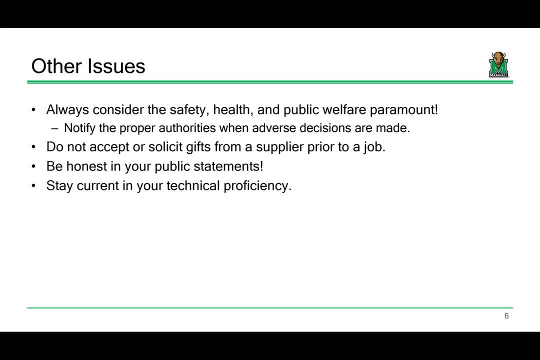 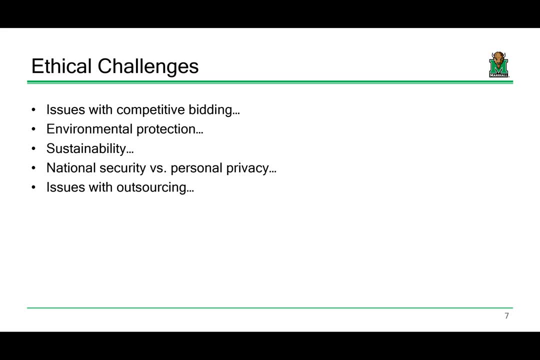 client good and does the engineering community good, as well as the public. make sure that you stay current in your field. here are some what I would call ethical challenges. we might be straying a bit beyond what is right for content for the FE exam. however, I can't help but mention some of these points because I think it might lead to a more fundamental understanding of ethics on your part. 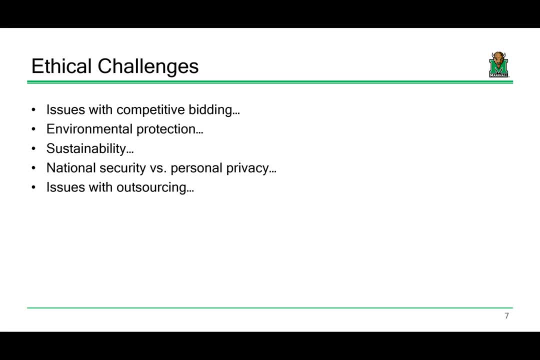 Some of these issues. we are starting to venture into gray territory. what is right versus what is wrong? Everything I've been talking about before is pretty cut and dried. It's pretty yin and yang: either one choice or the other. We're starting to get into gray territory here. 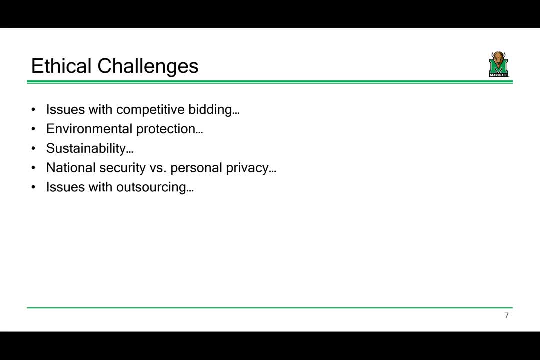 Maybe if you start doing some research and looking into some of these ethical issues, you'll start to gain a more refined understanding of engineering ethics. For example, there are some very significant ethical issues associated with competitive bidding. What I mean by that is, let's say, I'm an engineer and you're an engineer and we're both bidding on the same job. 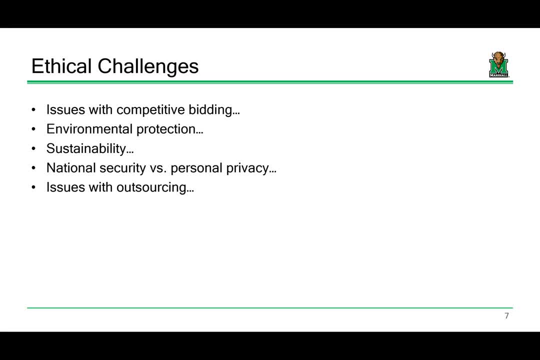 Well, that process, by its very nature, forces you and I to try and produce the lowest bid possible. Well, by that nature, that process can lead to you and I potentially wanting to cut corners, And this has been litigated upon. 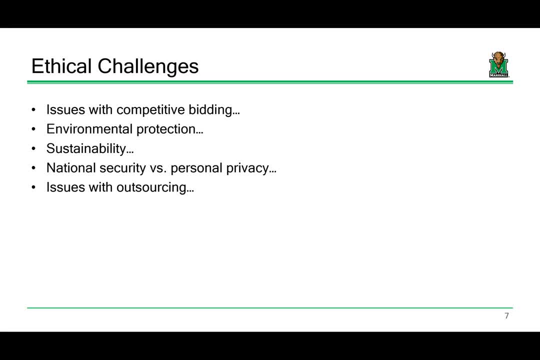 It's even gone all the way to the Supreme Court on issues like this And the way that the Supreme Court ruled- and there's reasons why competitive bidding really isn't mentioned- And many codes of ethics, is that the Supreme Court- I guess the best way of putting it is- they're not requiring competitive bidding. 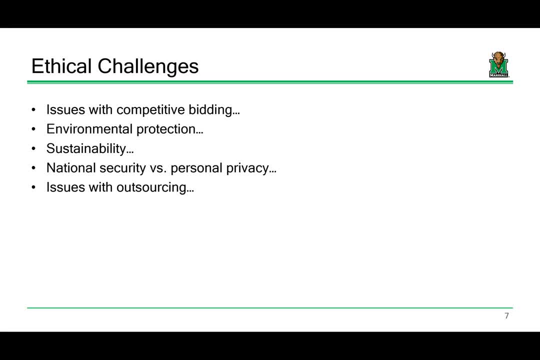 They're basically forbidding a prohibition against it, Like they're not encouraging it. They're saying you can't disallow it, And so competitive bidding happens, Like there's no way around it. It does happen, But there's some ethical issues there, because there's only so. 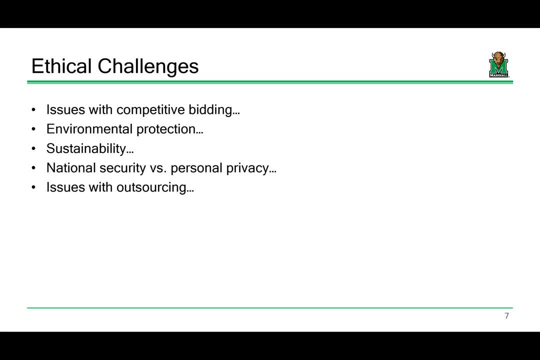 There's only so far that you can take that process. and then you start compromising your profession and compromising safety and so on and so forth, And then you start to get into ethical issues like environmental protection and sustainability. You know what responsibility do you have to the client versus the public, versus the environment? 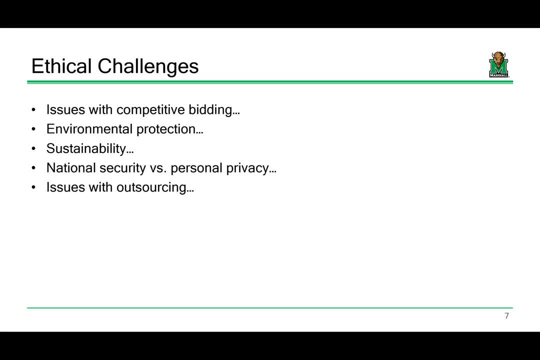 What about when you're designing something in the interest of national security versus personal privacy? I'd say one of the questions I always ask students and I always get very, very polarizing answers- is: is it ethical for an engineer to design a gun, to design a weapon? 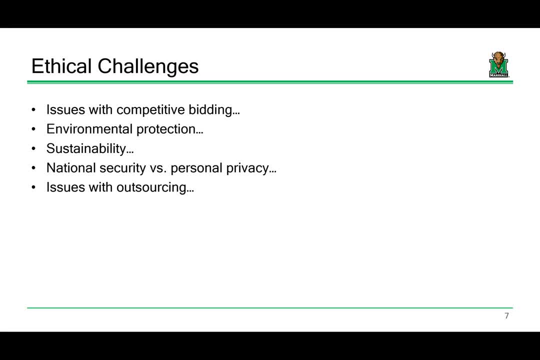 You know you're acting on behalf of your client, but then again you may be designing an instrument that will be used to potentially kill somebody. And so if your interest is to maintain the safety, health and welfare of the public, and yet you're designing an instrument of potential death, is that ethical? 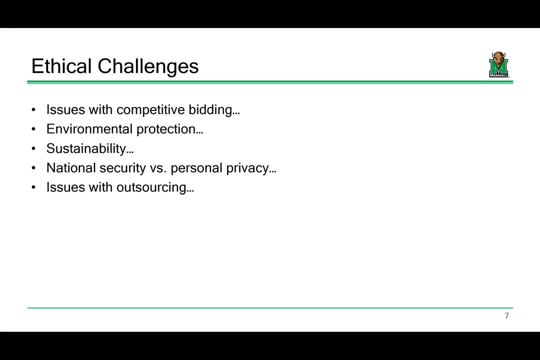 And so it really. you know, it's almost like that question in and of itself could cause any potential student to start pouring through codes of ethics and articles to try and understand it, And by doing that you'll gain a much more deep understanding of engineering ethics than by just reviewing a few problems on the FBE exam. 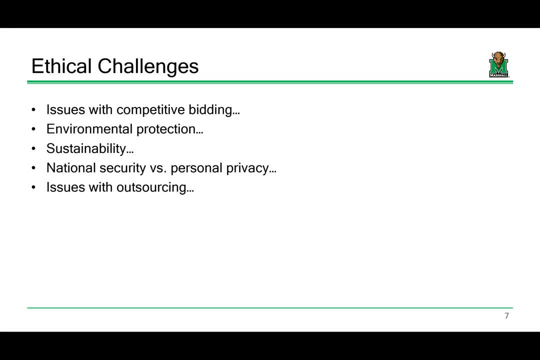 And so I really think that's, That's That there are some ripe areas of study there. Another potential ethical challenge- and I'll sort of close with this- is the issues with outsourcing work. Sometimes it's called offshoring, You know, instead of designing within your organization or within your firm, or a simple way of thinking about it, even though it's not really. 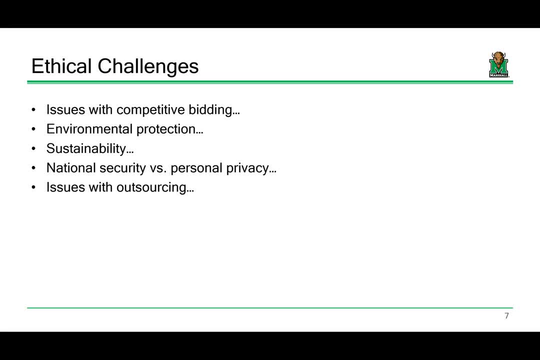 From an engineering perspective. I'm not really talking about outside the country, But it's. It's easy to discuss it in this fashion: Instead of using design services in the United States, maybe you just outsource that work to a firm in another country. 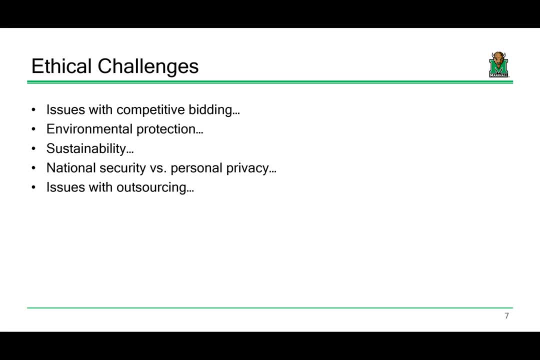 And you do that because it will save you money and save you resources. Well again, there are ethical issues with that. Not even so much from a public safety and welfare standpoint. I think that's an easy argument to make, To say: well, you know. 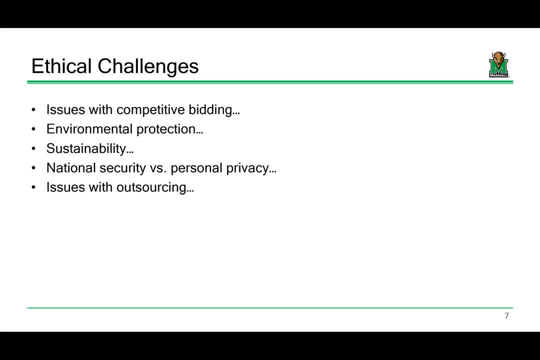 You can't outsource something to save money if it's going to compromise public safety. I think that's easy. What's more difficult is when you start doing that, are you outsourcing the responsibility as well? You making that decision to outsource that work? 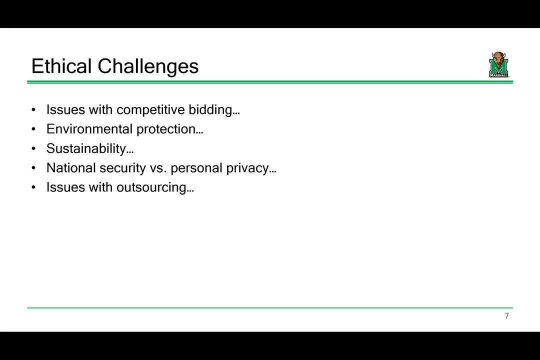 Who's responsible if things go wrong? Is it you or is it the outsourced client? if they're outside your sphere, Yeah And the The out-of-the-country analogy works quite well, because they might even be outside the laws of your given region, of your given area. 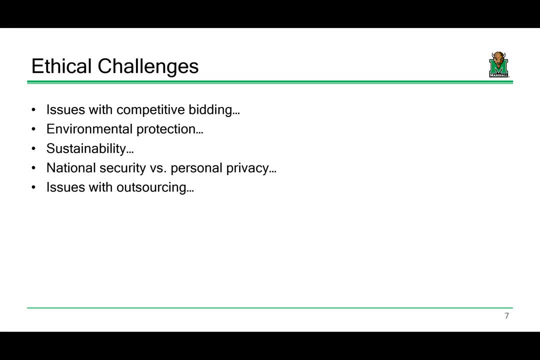 So there are some very significant challenges here And this one slide. you can take any one of these bullet points and by researching it you'd be studying this concept, in my opinion, far better than you would by just doing some ethics problems. 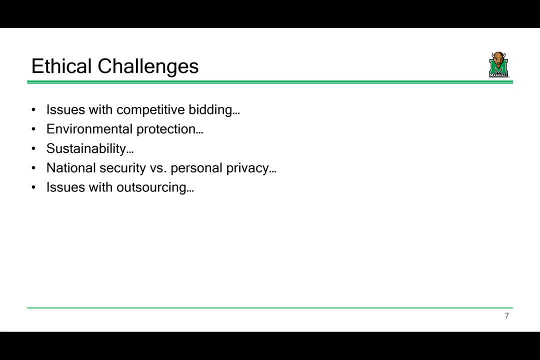 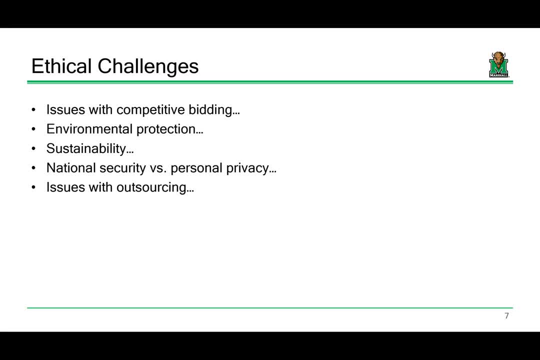 And come from a studying perspective, Because it's not like math or chemistry or physics, where you learn by doing problems. The more that you do, the better you get at them. With ethics, sometimes the problems are so disparate that each problem is a case-by-case basis and there's no real learning involved. 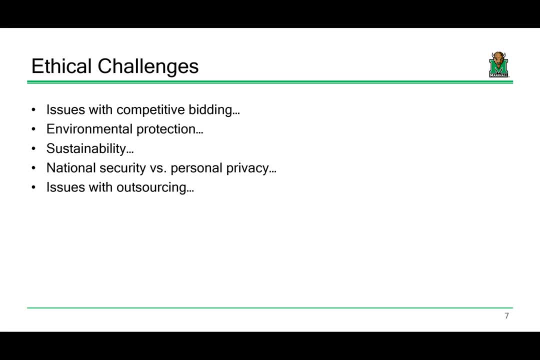 And so I think the learning comes from taking a complex ethical issue and researching it, and studying it and trying to form your opinion, And by doing that you'll be. You're viewing these codes And hopefully you all do that. I will post a quiz online with some ethical questions just to give you that experience. 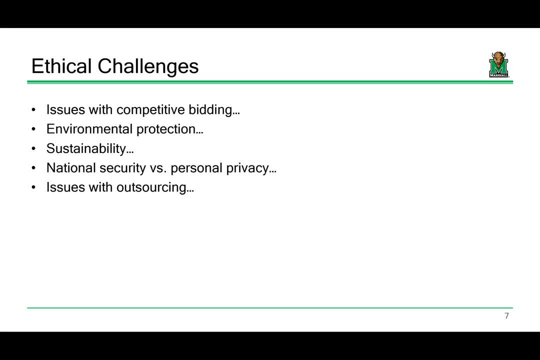 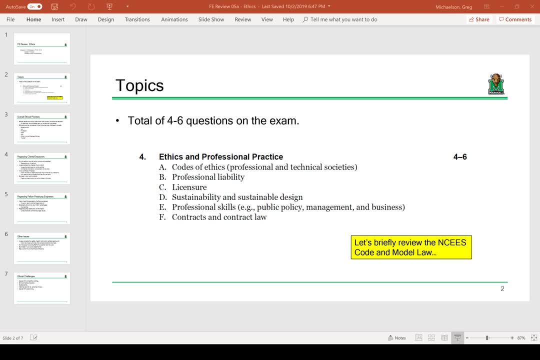 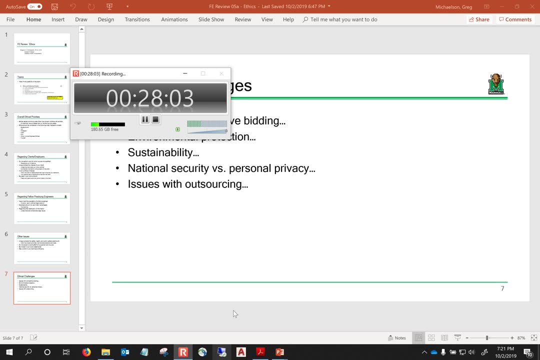 But I do think that you should pour into this a little bit, because there's some really interesting potential avenues to look into. That's all I have for this lecture. I'll be posting a lecture later on on looking at computational tools. That's all I have.